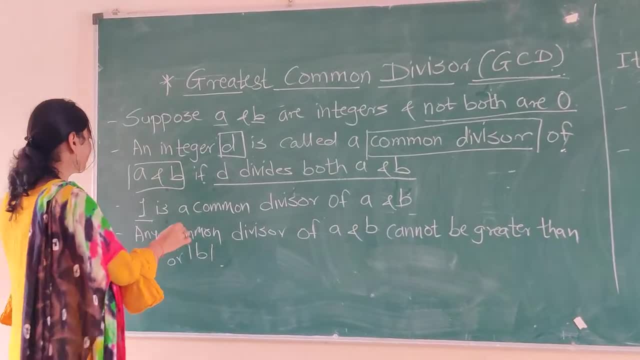 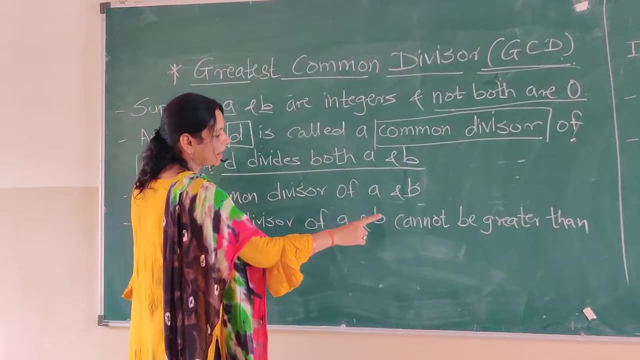 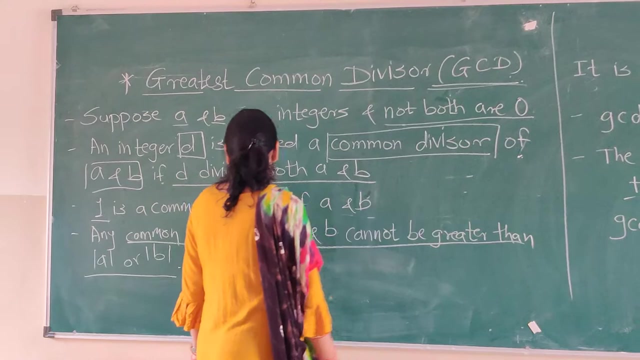 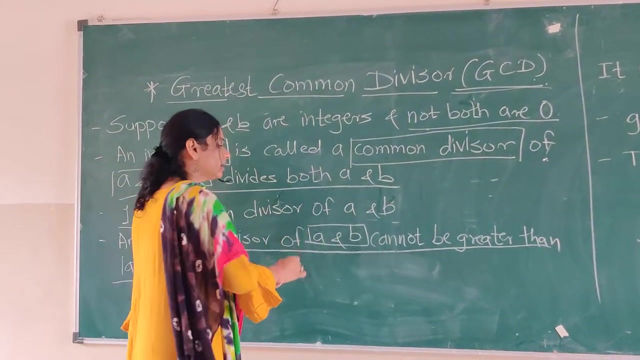 Okay, Okay, Whatever may be the number, because 1 will be, but 1 will be the common divisor of any integer. Any common divisor of A and B cannot be greater than 1 of A or 1 of B. Keep in mind that any common divisor of A and B can't be greater than A and B, always. That is the main condition. 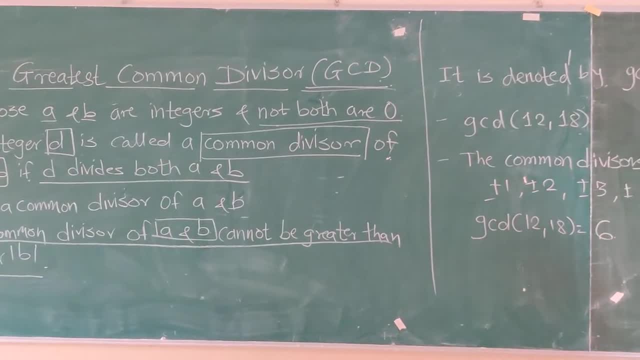 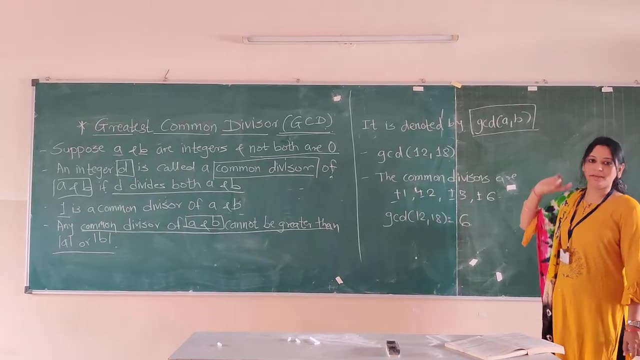 Now how GCD is denoted. So GCD is always denoted by this, That is, GCD in bracket A and B. So we will see the example. So, in short, this is GCD, What it is, nothing but greatest common divisor. 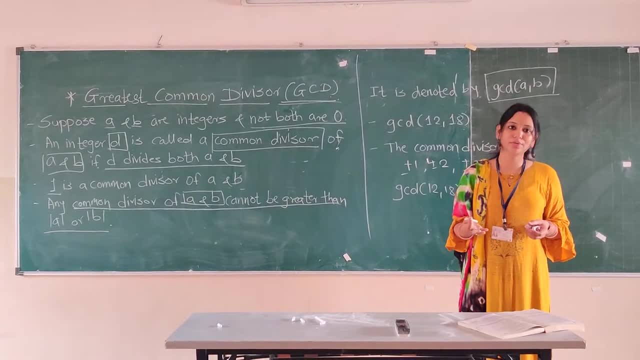 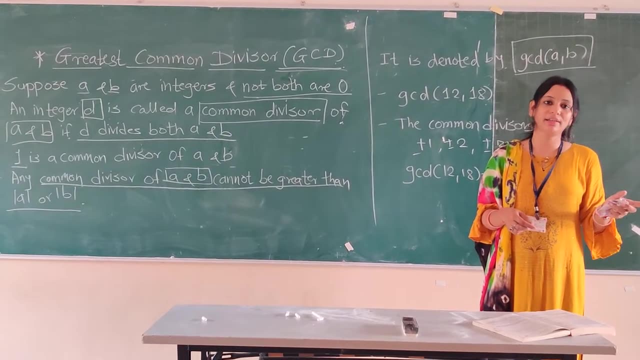 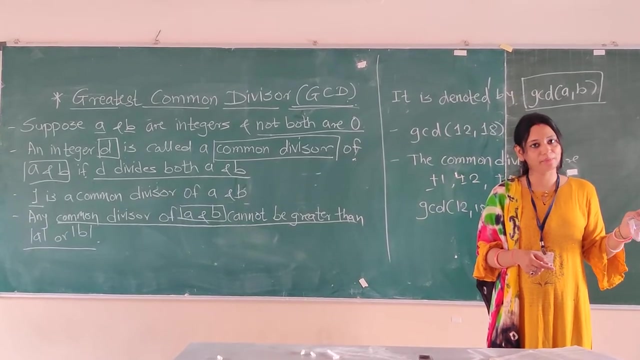 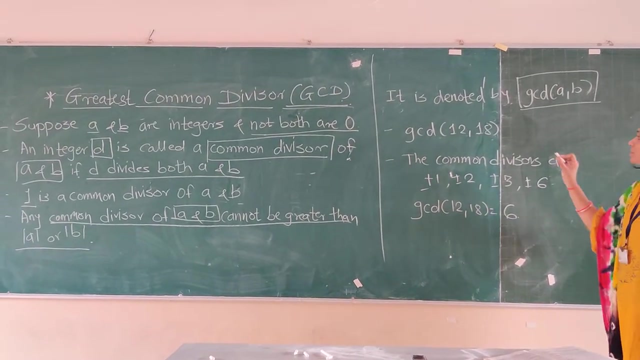 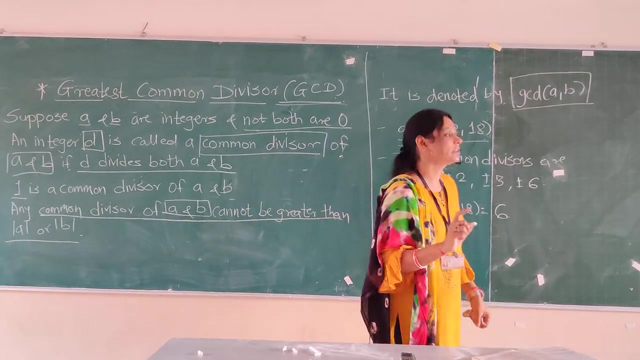 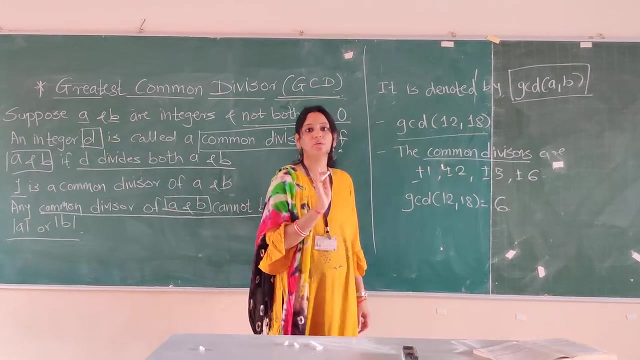 Suppose we are having the integers which are the non-zero integers. Then suppose we are having the third integer and the third integer is able to divide A and B integers, Then that is the common divisor. Then whatever common divisor which we are having, in that the greatest number is called as the greatest common divisor, Okay, So suppose we are trying to find GCD of 12 and A and B. So what will be the first step? The first step is: we can see it is non-zero number. Okay, So we will find out the common divisors first. Which are the common divisors? 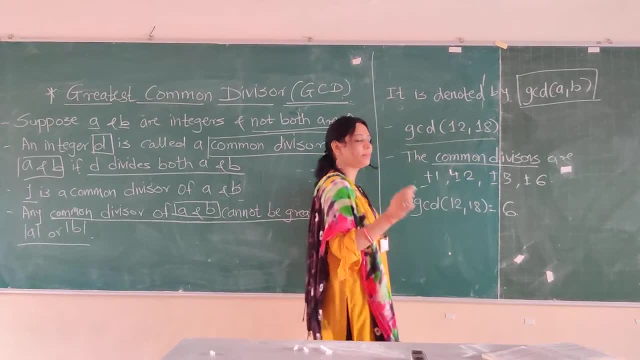 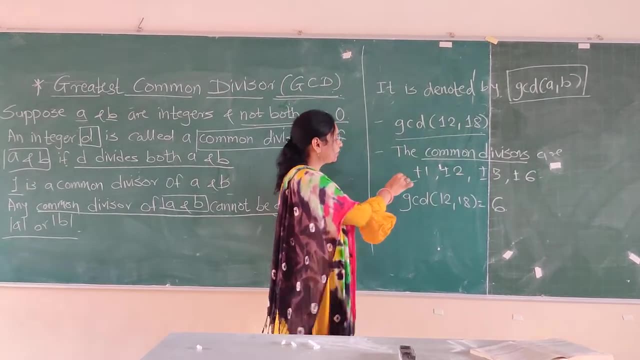 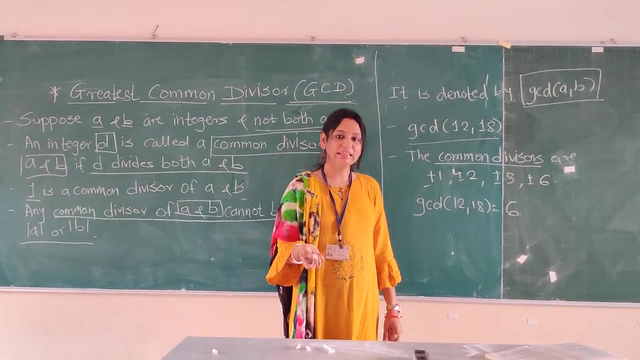 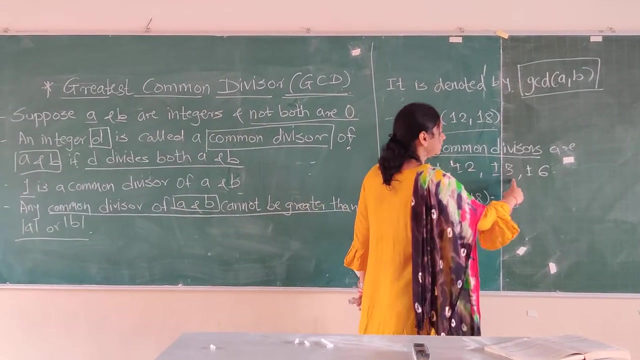 So 12 and 18, the common divisors are 1,, 2,, 3 and 6.. Now I have taken both the values, positive and negative, because the numbers can be divided by the positive number as well as the negative number. So the common divisors for 12 and 18 are 1,, 2,, 3 and 6.. And we are trying to find out GCD. 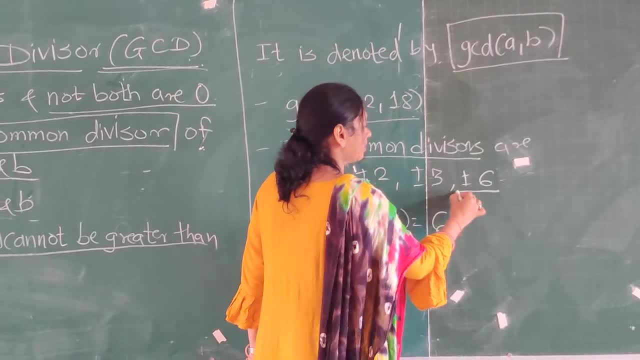 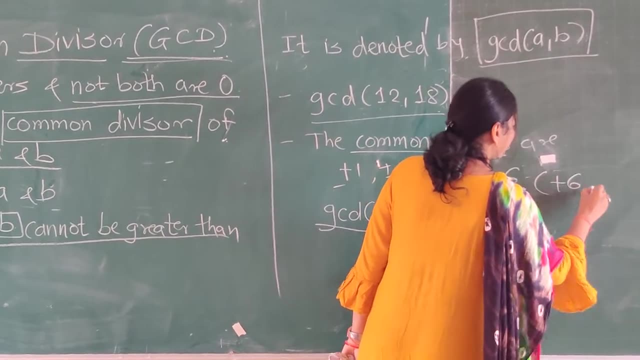 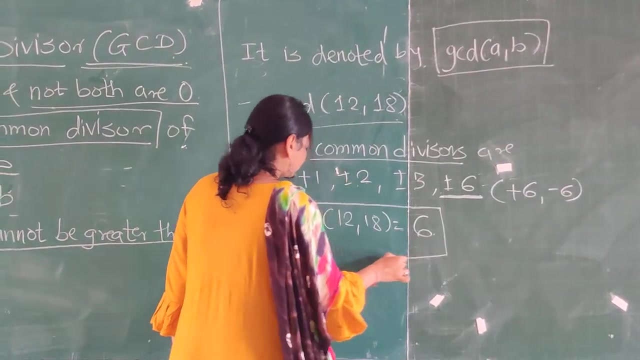 So which is the greatest common divisor here? This Plus minus 6.. And in plus 6 and minus 6.. Which is greatest Definitely positive integer, That is nothing but common divisor. That is, GCD of 12 and 18 is 6..